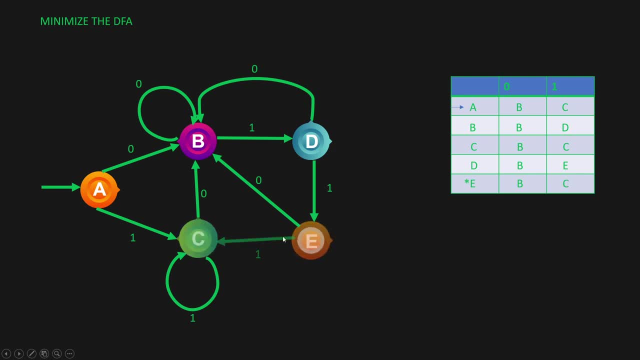 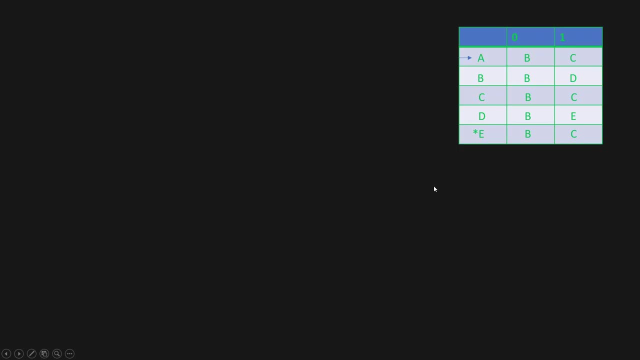 0.. You go to state B And you are in state E. you get input 1, you go to state C. So this is our transition table for our DFA. Alright, now, with this transition table, we will create minimization or we will perform minimization by creating a minimized transition table. 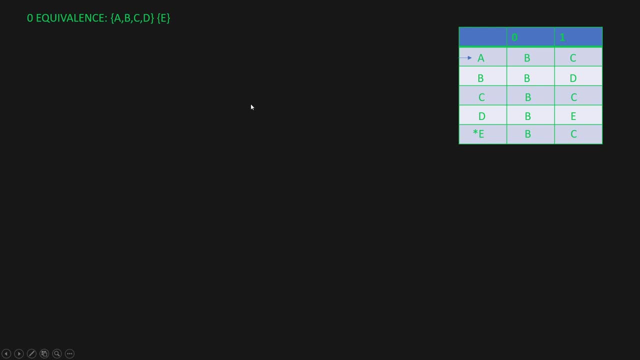 Alright, so first, what we will do is we will write zero equivalence, So minimization through equivalence. So what is zero equivalence? We have to divide all these states in two groups: One group of final states and one group of non-final states. 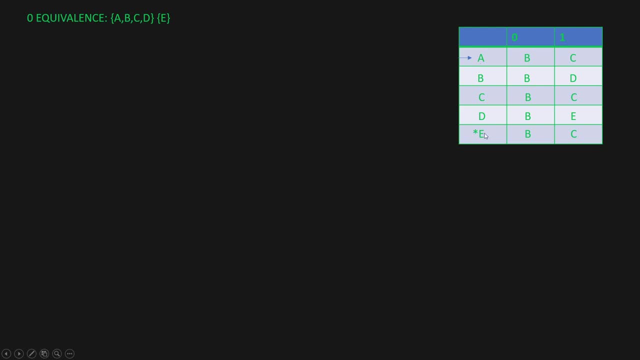 So, as we can see, A, B, C, D, these are non-final states and E is the only final state. That is why I divided it into these two groups. Now, the one equivalence is, you have to see, based on the output, which, whether the output lies in the same group as the input or not. 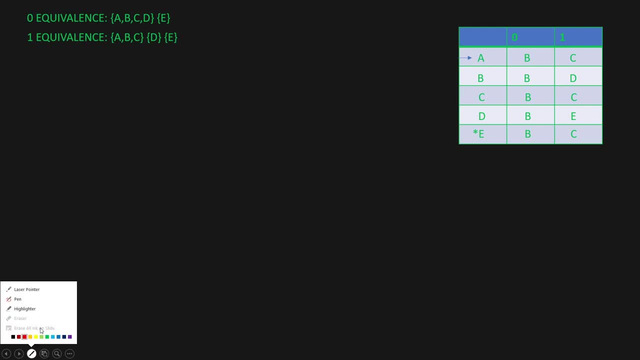 So what does that mean? So let us say, let us use the pen, okay, green color, Alright. So let us say we have to compare A and B and check whether they are one equivalent or not. So let us say you have state A and state B And when you get input zero in state A, you 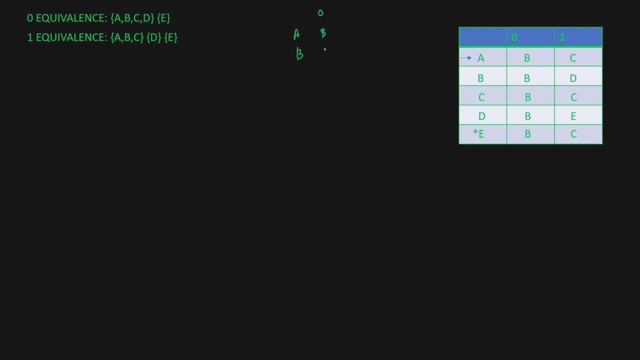 go to state B, And in state B also, you get input zero. you go to state B. What about input one? You get input one In state A, you go to state C And in state B you go to state D. Now are C and D part of the same group over here? No, C and D, sorry. C and D they. 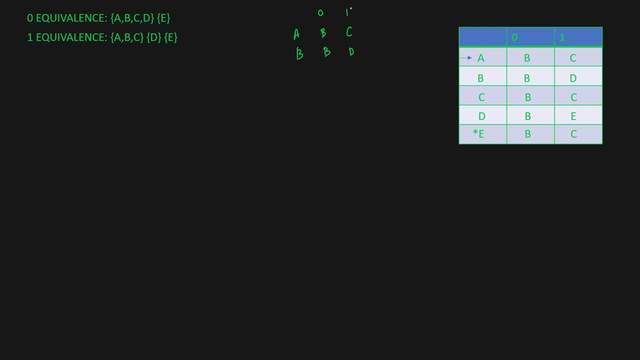 are part of the same group. So that is why one getting the inputs, that is same input one- C and D are present in the same group. That is why A and B are one equivalent. A and B are one equivalent. 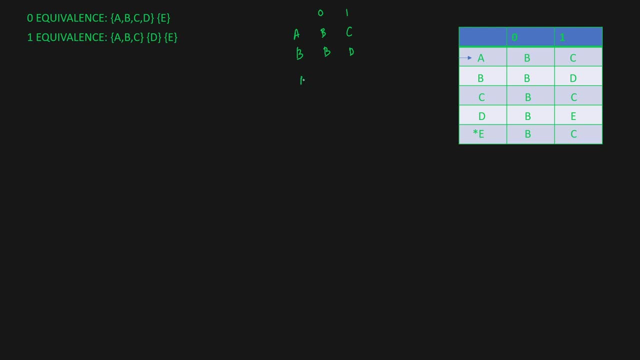 What about A and C? So let us say you have got A and C. Let us compare directly. Okay, So let us say you get input zero in C, you go to state B, And you get input one, you go to state C. So is C and C and B and B part of the same group? Yes, it is part of this. 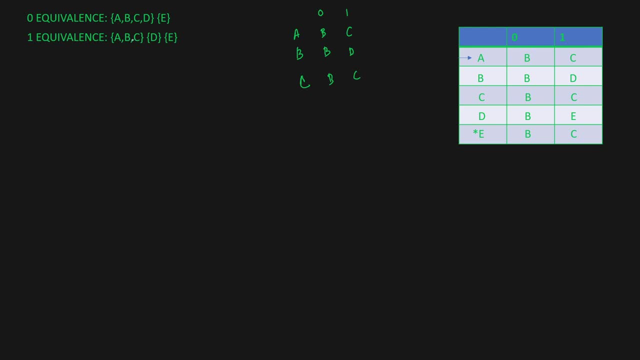 same set. So that is why A, B, C, these are what One equivalent. What about D? We have to compare D now. So let us say D, we will compare it with C itself. Okay, So in D you. 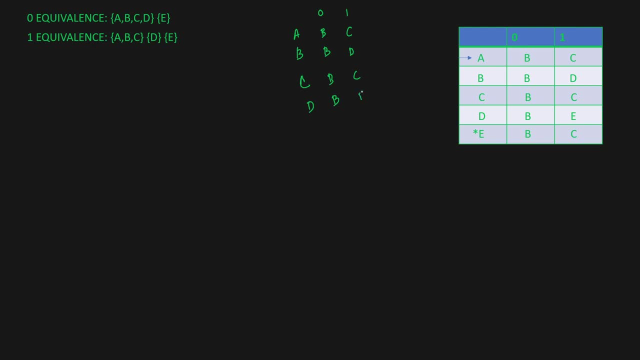 get. on input zero, you go to B, And on input one, you go to state E. Now are C and E part of the same group? No, they are not, Because, as you can see over here, C is in this set, E is in this set. That is why D is not part of this set. That. 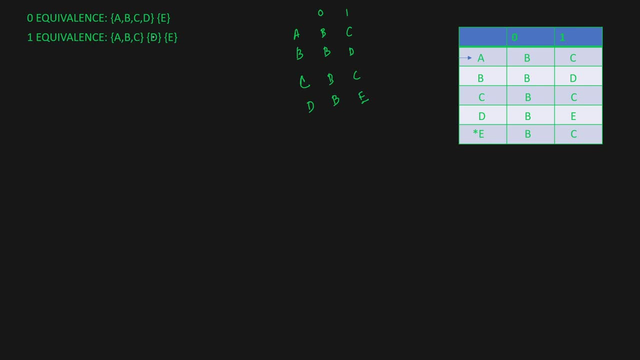 is why D is not one equivalent with A, B, C, So you create a separate set for D, and E was already present in the separate set. Now we will check for two equivalents. Now, what is two equivalents? Same process we will apply and we are going to compare them again. 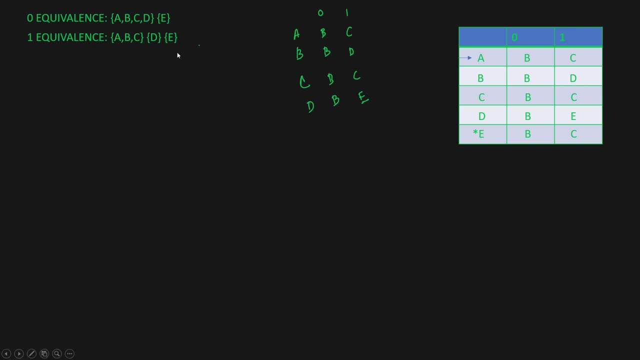 Okay, Now just a second. Yeah, Okay. So two equivalents means we have to compare A and B. On getting zero, they are both having output as B And on getting input, one. one is having C, one is having D. Now is C and D present over here in the same set? No C and D are. 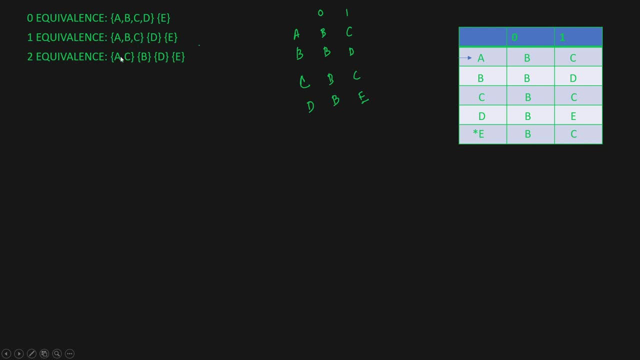 not present in the same set. That is why A and B are not two equivalents. That is why we create a new set for B over here. Okay, And A and C are two equivalent. Why? Because they are getting the same outputs, B and C- in the same input. So for input zero, A and 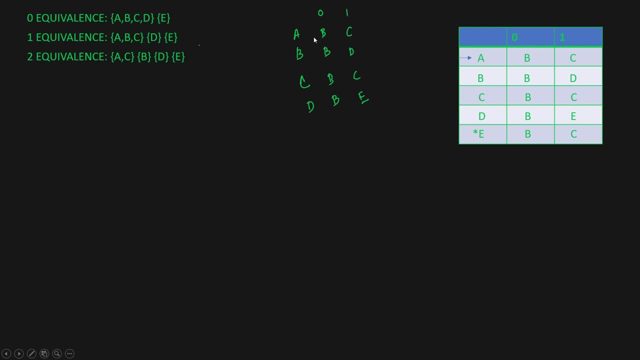 B are having the same output B And for input one, both of them are having the same output C. Okay, That is why A and C are two equivalent. Now we will perform the same thing with three equivalents. We will check for the same thing And we are going to get 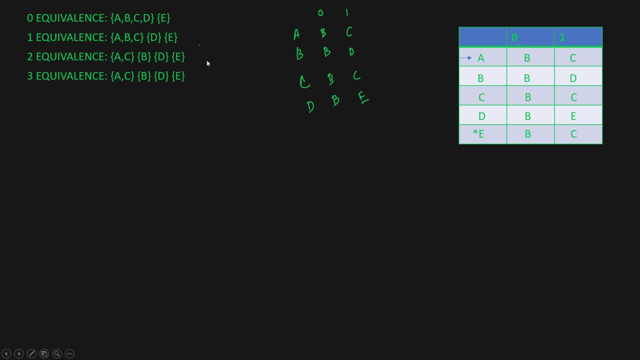 these three sets. So when we get two equivalents back to back same, then we stop over here. Okay, Now what we will do is we will perform or we will create a new transition table with these combined two states over here, That is, A and C. We combine them and form a new. 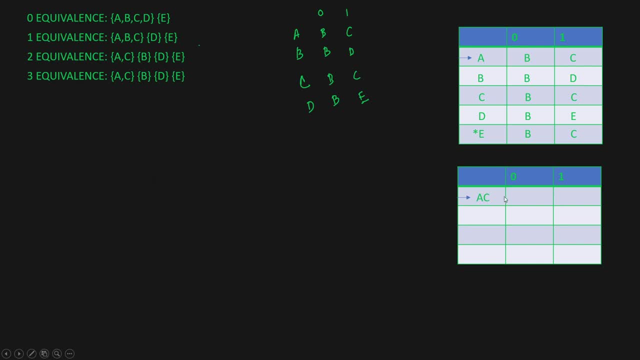 state called A C, Okay. So first state is A C. In getting input zero in state A C, we are going to go to state B. Okay, And on getting input one, we are going to go to state C. But there is no such state as C, It is A C. 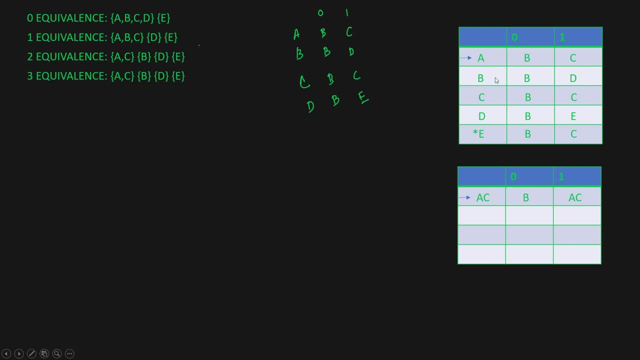 That is why we write it as A C, Because we have combined A and C. What about state B? You get input zero, you go to state B, And on getting input one, you go to state D. What about state C? There is no state C. We have already written for state A C. Okay, Next. 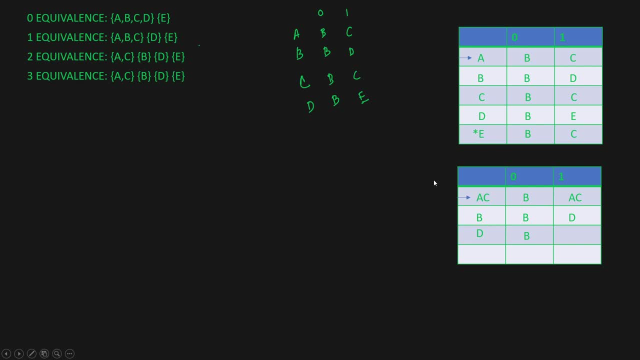 is state D. On getting input zero, you go to state B. What about state E? You get input zero, you go to B And you get input one, you go to state C, But there is no state C, You go to state A, C over here. Okay Now, based on this, 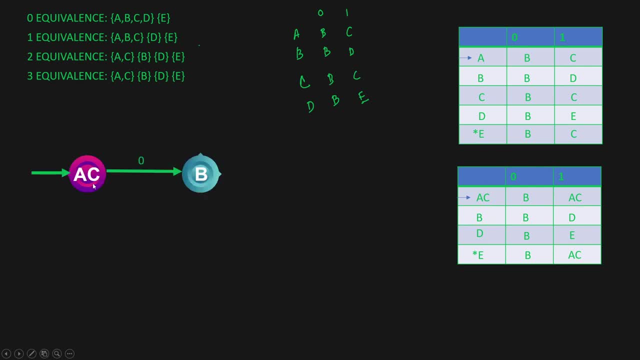 new transition table. we will draw our DFA diagram. So we have got first starting state A C. You get input zero. you go to state B, Correct, And you get input one. you are going to state A C, First part done. What about state B? 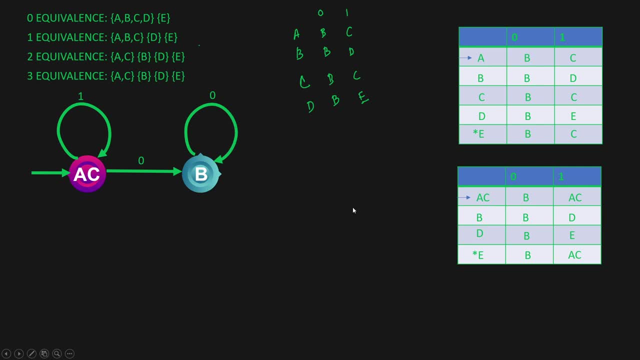 You get input zero. you go to state B itself. You get input one. you go to state D. Okay, What about state D? You get input zero. you go to state B- Correct, And you get input one. you go to state E. In state E, what happens? You get input zero. you go to state B And 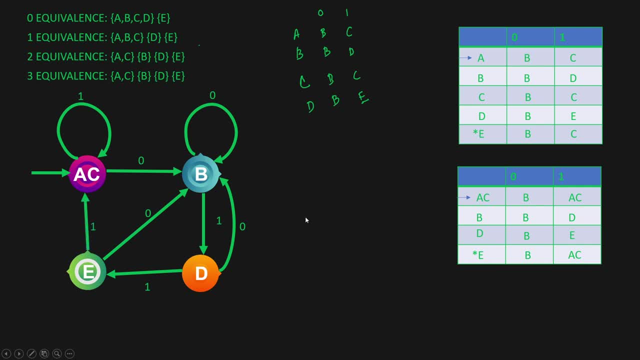 you get input one, you go to state A, C. So this is how we minimize our DFA. So I hope you got this concept. If you have any queries, feel free to ask me in the comment section below. Thank you very much. 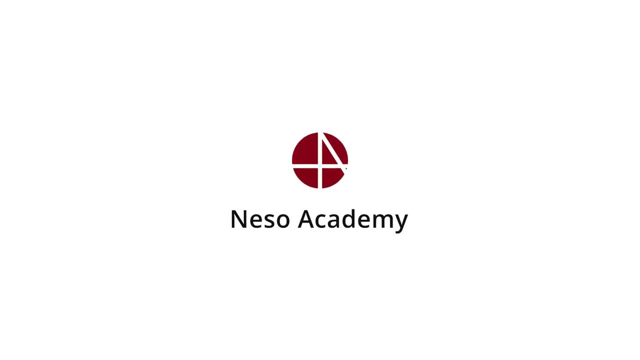 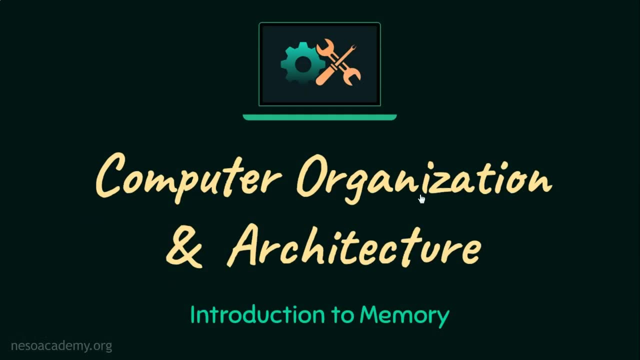 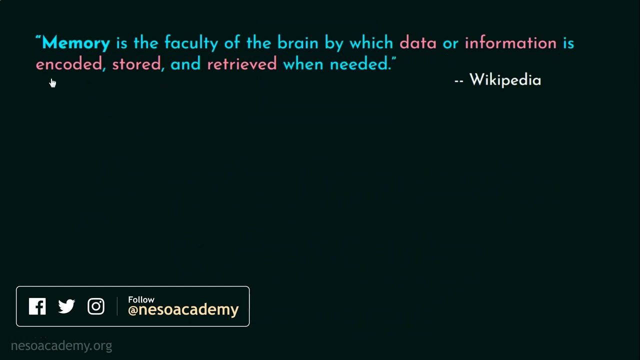 Hello everyone, welcome back to this wonderful journey of computer organization and architecture. In this session we will be focusing on memory, So let's get to learning. Wikipedia states memory is the faculty of brain by which data or information is encoded. 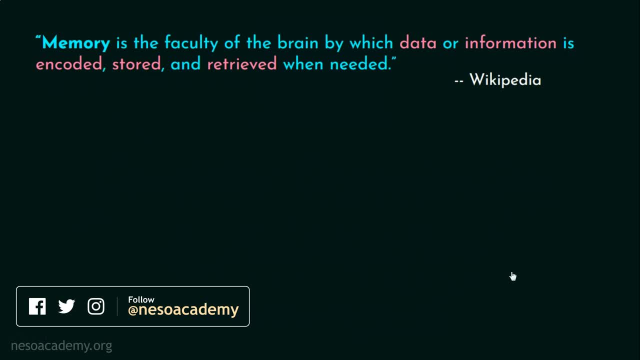 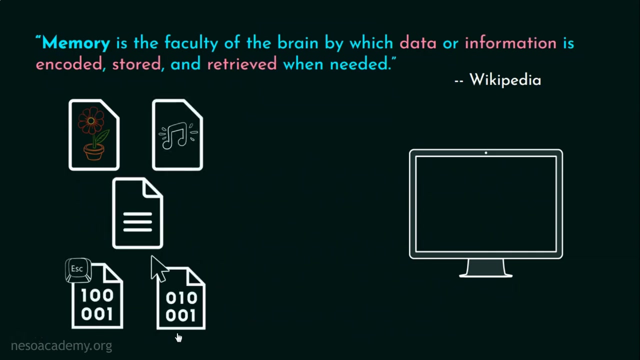 stored and retrieved when needed. Similarly, in case of computers, memory, which was initially termed as store, plays a similar role. Everything, be it an image, an audio file, a text file or instructions for a key press or a mouse click, if that is stored in the computer memory. 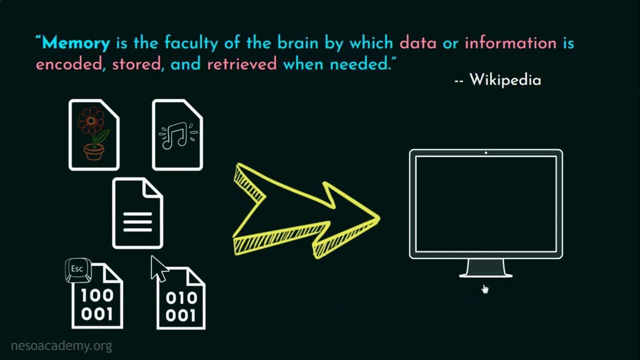 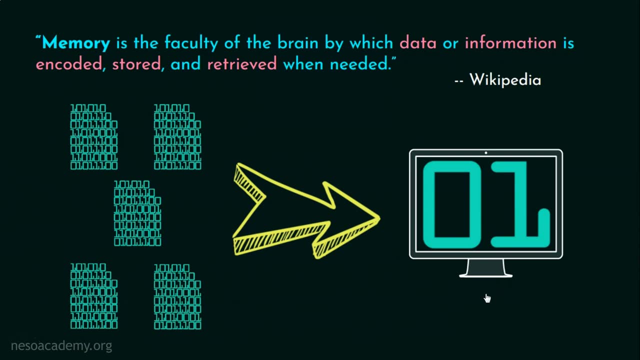 it's actually encoded as bits. Basically, each memory cell can have either 0 or 1, and all these are comprised of a memory cell, Millions of bits, and processed by the processor, the brain of the computer. So we might think that having a single large memory unit is the solution to this situation.